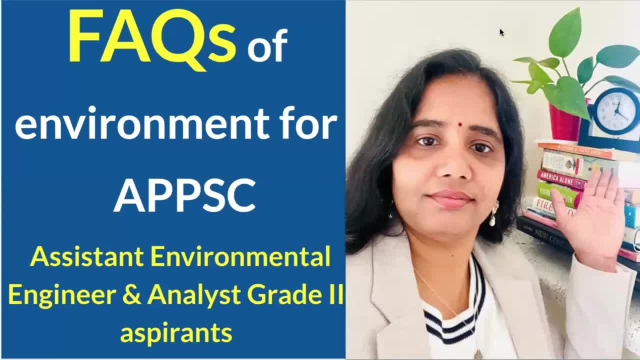 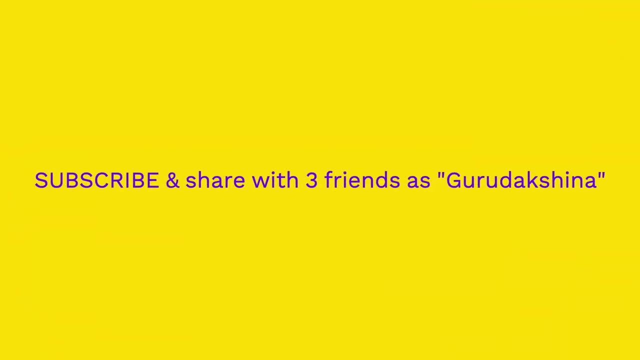 Hello, I am Dr Annapurna Singh and this is Frequently Asked Questions of Environment for Andhra Pradesh Public Service Commission, Assistant Environmental Engineer as well as Analyst Grade 2 Aspirants. I will use both English and Hindi in this video so that everybody can understand. 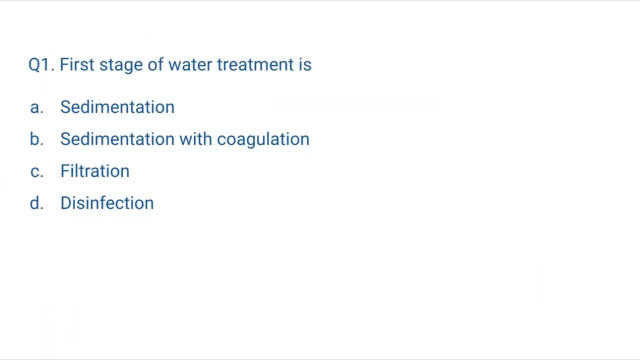 Okay, question number one. First stage of water treatment is A Sedimentation, B Sedimentation with coagulation, C Filtration, yet D Disinfection. So the first stage of water treatment is A Sedimentation, B Sedimentation with coagulation, C Filtration, yet D Disinfection. 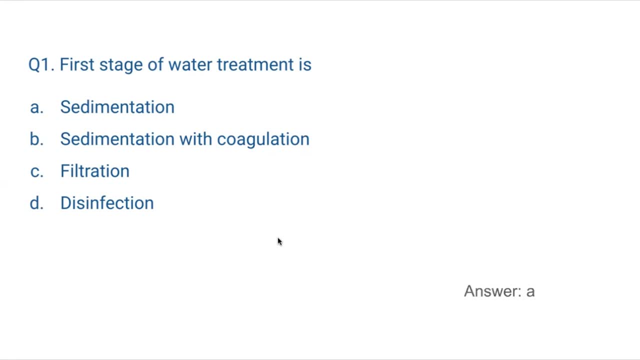 The correct answer is A Sedimentation. First there is screening, then A Sedimentation, then A Sedimentation with coagulation, then A Filtration- In Filtration all the flocks are removed- and then A Disinfection. 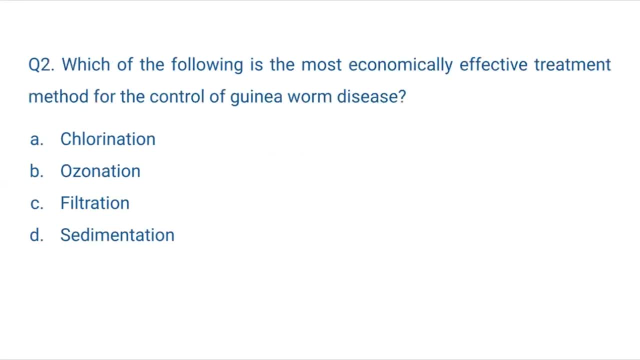 So these are the stages of water treatment. Let's move on. Question two: Which of the following is the most economical? Which of the following is the most economically effective treatment method for the control of Guinea Worm Disease? Guinea Worm Disease is clearly caused by pathogens. 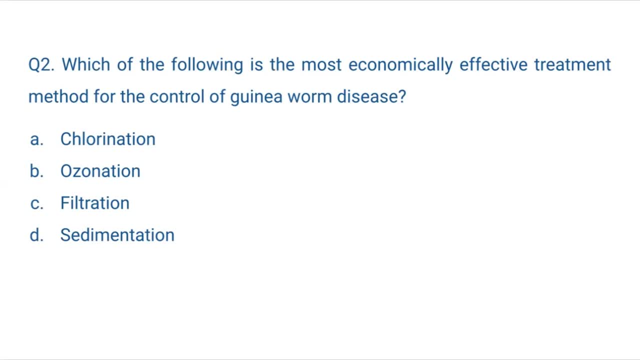 So Guinea Worm Disease is a pathogenic disease And the most economically effective treatment, the cheapest treatment. what will happen? Chlorination, Ozonation, Filtration and Sedimentation. So Sedimentation is not enough. Sedimentation is not enough. 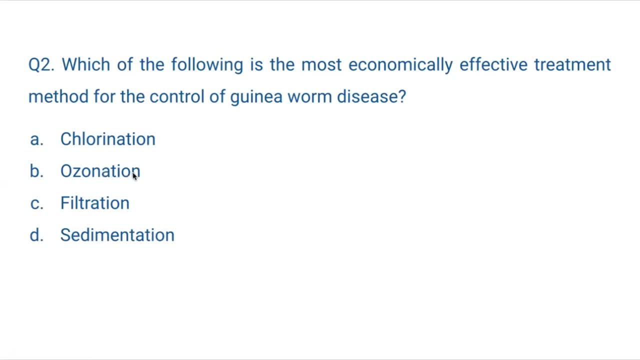 And Ozonation is an expensive treatment. Ozonation is expensive. The two options are Chlorination and Filtration. Both of these are cheap methods. You don't have to do anything else, Just filter the water and it will be free from Guinea Worms. 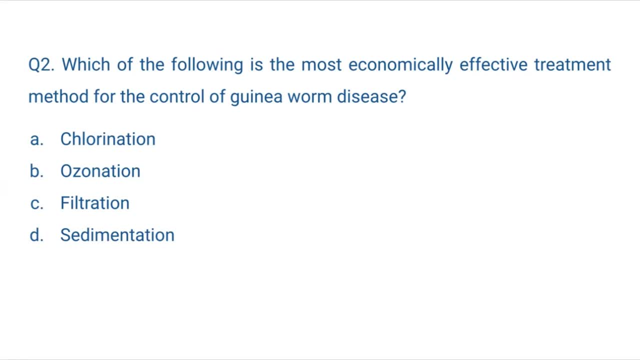 So if you want to do filtration, then simply, if you don't have chlorine, if you don't have anything, if you don't have home water, then you can filter it. then it will be free from Guinea Worms. The easiest method is Filtration and after that Chlorination. 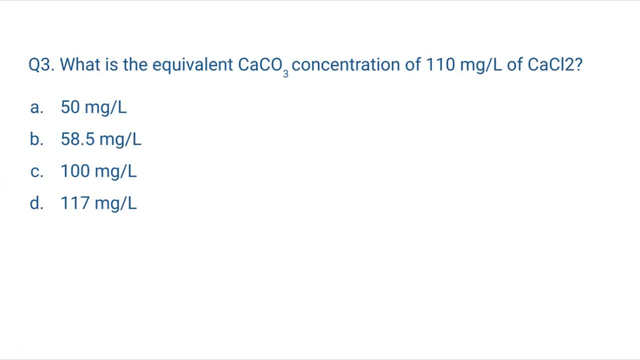 Question three: What is the equivalent calcium carbonate concentration of 110 mg per litre of calcium chloride? Okay, So the concentration of calcium chloride is 110 mg per litre and it is asked that what is the equivalent of calcium carbonate? So we will first find out the equivalent of the 110 mg per litre of calcium chloride and then we will do it in terms of calcium carbonate. 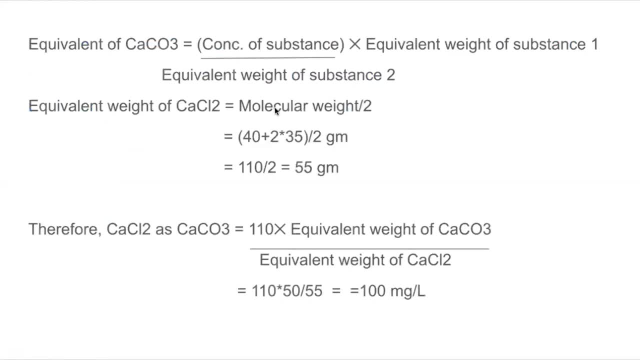 So first understand the question. The answer is C. Now how will it come? Equivalent of calcium carbonate is equal to concentration of substance into equivalent weight of substance, one divided by equivalent weight of the substance, two. So equivalent weight of substance two, which is calcium chloride. 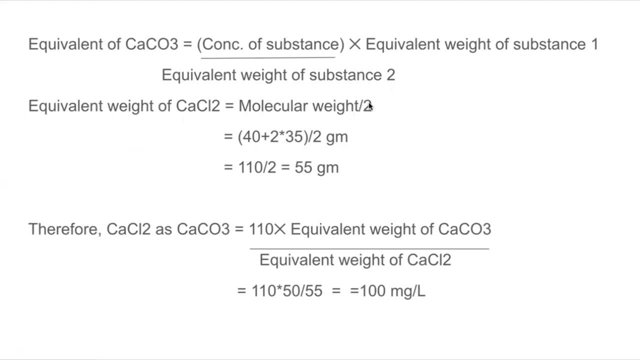 So equivalent weight of calcium chloride. what will happen? Molecular weight divided by two, which is valency? Okay. So molecular weight of calcium chloride is calcium, the atomic weight is 40, then chlorine, the atomic weight is 35.. 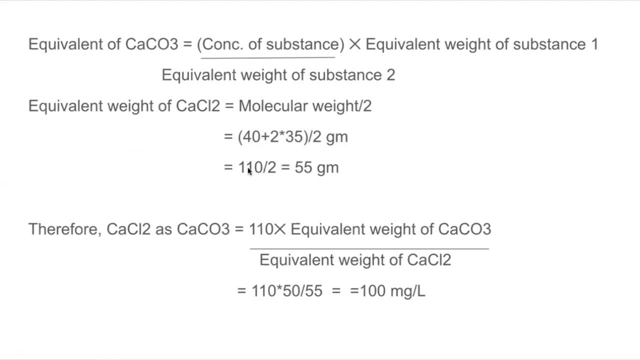 So 40 plus 2 into 35, divided by 2 is equal to 110. by 2 is equal to 55 g. So equivalent weight of calcium chloride is 55 g. Therefore calcium chloride as CaCO3 will be 110.. 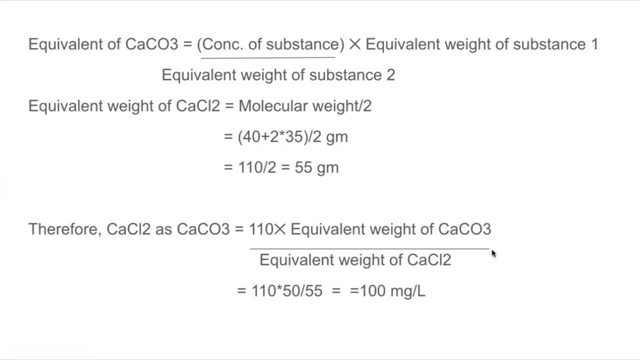 That is, it will be 110.. That is, it will be 110.. So the concentration of calcium chloride into equivalent weight of calcium carbonate divided by the equivalent weight of calcium chloride, So 110 into 50, equivalent weight of calcium carbonate, 50 is there, divided by 55, which we have calculated here, is equal to 100. 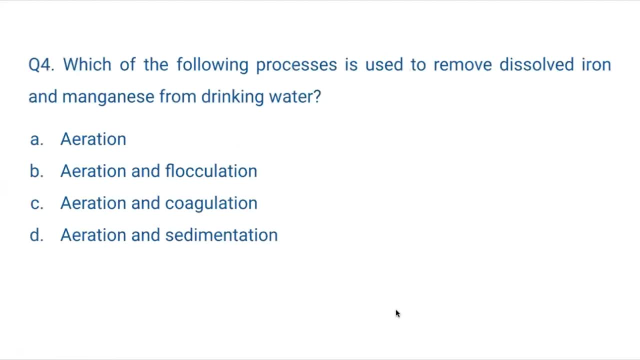 That is the answer. Okay, Question 4.. Which of the following processes is used to remove dissolved iron and manganese from drinking water? Now, which of these processes is used to remove dissolved iron and manganese? Arration, arration plus flocculation, arration and coagulation, or arration and sedimentation? 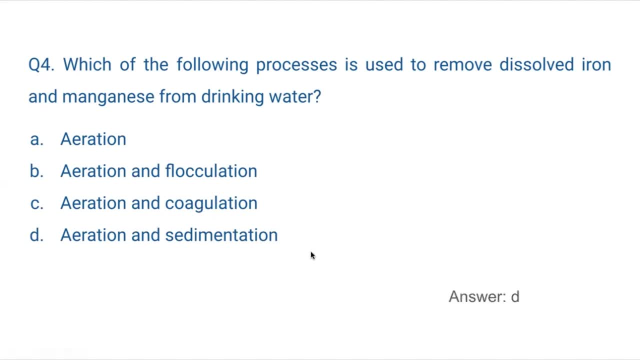 The correct answer is D, Arration and sedimentation. When you aerate the water, it oxidizes the iron and manganese present in it. The oxides are heavier, they settle down at the bottom during sedimentation and then the clear water is removed from the top. 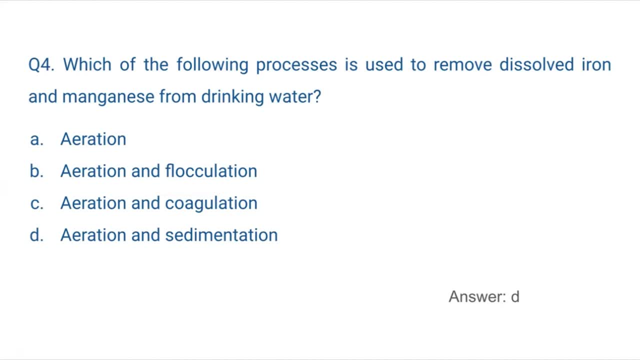 The answer will be D, because you have added air oxygen and aerated the water, so iron and manganese change to their own oxide. They are heavy. These oxides are heavy and then they settle down during the sedimentation process and then the clear water is removed from the top. 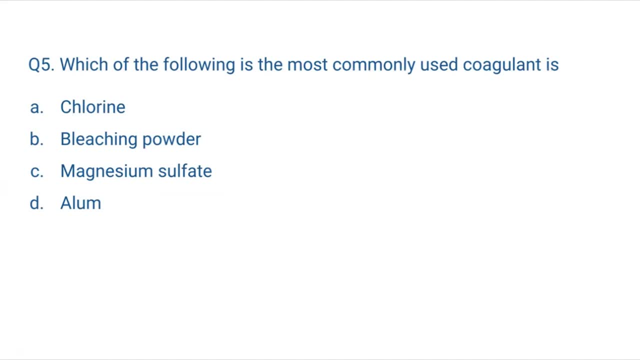 Question 5.. Which of the following is the most commonly used coagulant? Which is the most commonly used coagulant? Chlorine? Chlorine is not a coagulant. Chlorine is a disinfectant. Bleaching powders. 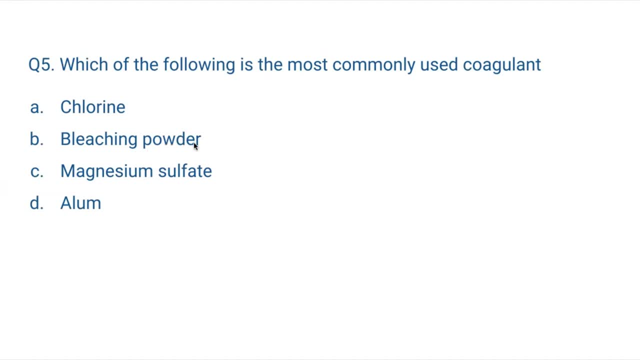 CaOCl2.. This is also not a coagulant. It's a disinfectant. Magnesium sulfate and alum: These two are coagulants, And alum means phytkari. It's the most common coagulant. 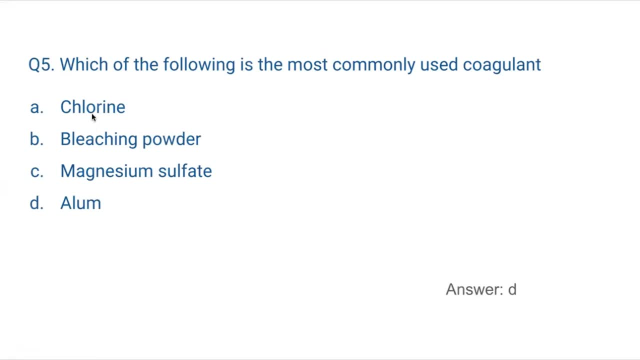 So alum is a phytkari. It's the most common coagulant. Chlorine and bleaching powders are coagulants, not disinfectants. The answer is D, Question 6.. Which of the following processes are necessary for removing suspended solids from water? 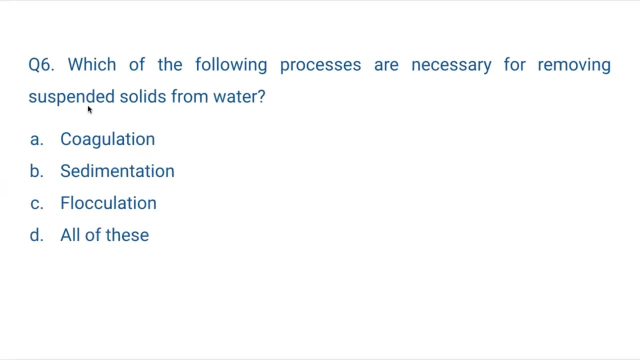 Which process removes suspended solids from water? A- Coagulation, B- Sedimentation, C- Flocculation Or D- All of them. Correct answer is D- All of these, All of these are correct. First of all, we add coagulant. 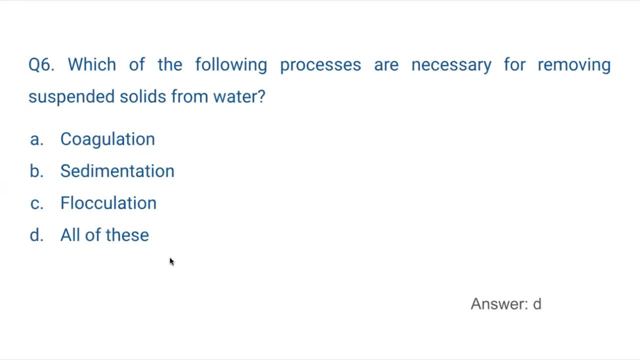 We add coagulation, After that we churn it, Flocks are made Flocculation, Then we sediment it, Sedimentation And finally clear water comes out from above and sediment stays at the bottom. So this is the whole process. 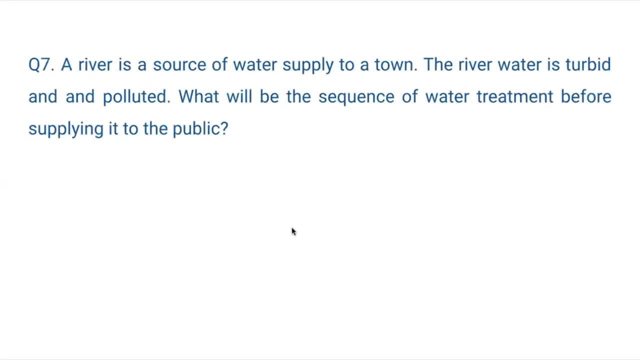 Question 7.. A river is a source of water supplied to a town. The river water is turbid and polluted. Correct answer is D. What will be the sequence of water treatment before supplying it to the public? A. There's a water source, a river. 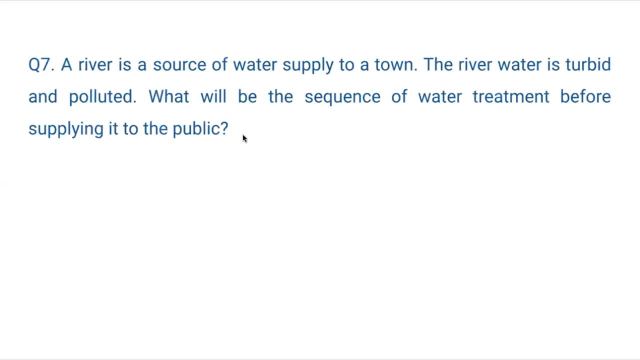 But the water in the river is dirty and crumbling. It's turbid and polluted. So what will be the sequence of treatment? If the water is dirty and you know it's polluted, You'll have to do a detailed treatment. Only disinfection will not be enough. 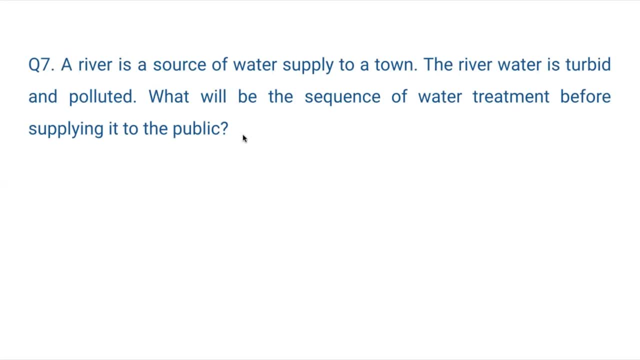 So if a source of water is visibly turbid, that is dirty and you know there are pollutants in it, That means it needs a detailed treatment and mere disinfection and supply management and supply management will not work. so the detailed treatment will be like this: screening first you have to pass the 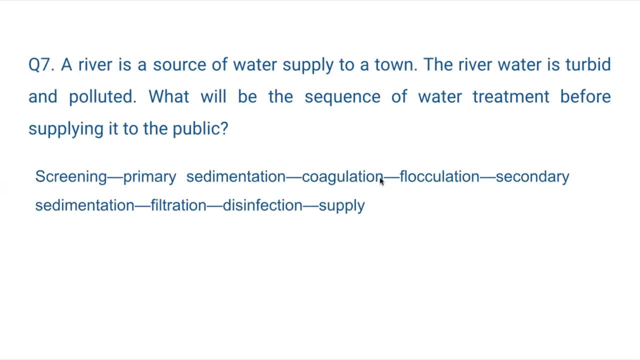 water to the screen, then primary sedimentation, then coagulation, adding coagulant which could be an alum, which could be alum. then flocculation to allow to form flocs, then secondary sedimentation- flocs will settle down. then you filter the water filtration and then you disinfect with chlorine. 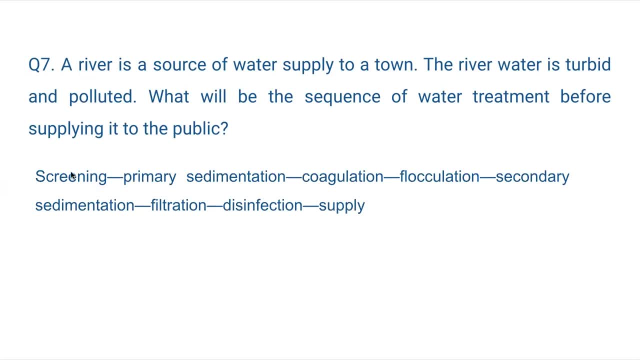 or leaching powder, whatever, and then finally supply the screening, then primary sedimentation, then coagulant will be added, coagulation, flocculation will be formed, flocs will be formed. then secondary sedimentation means flocs will be sedimented and then that water will be removed from above and the water which will come out from above after secondary, 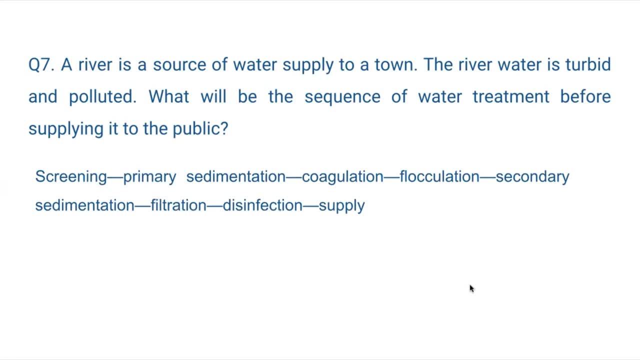 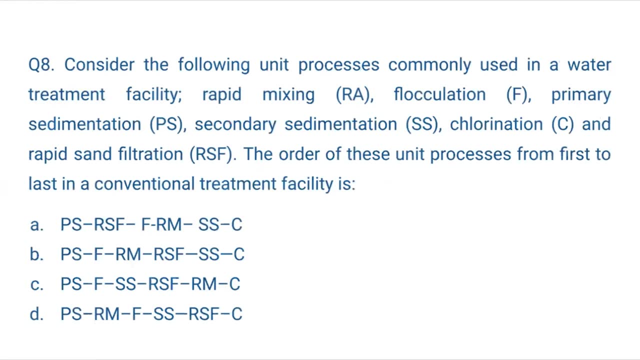 sedimentation. it will be filtered, disinfected and then supplied. okay, so this will be correct. treatment question eight current uh consider the following unit processes commonly used in a water treatment facility: rapid mixing, ra, flocculation f, primary sedimentation, ps, secondary sedimentation, ss, chlorination c and sap, rapid sat filtration, rsf. the order of these unit processes from first to 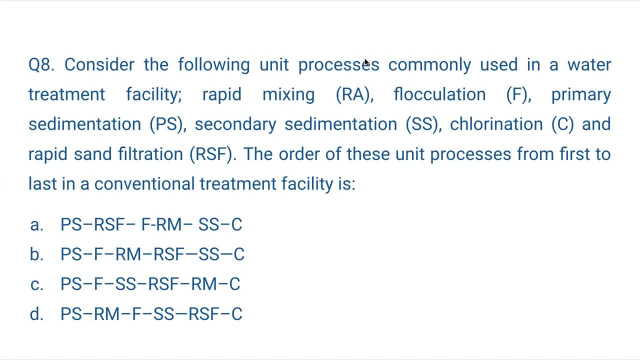 last in a conventional treatment facility is. these are the processes. we all know that the first step is primary sedimentation, we know that. and the last step is disinfection of chlorination. we know that. now primary sedimentation, then comes rapid mixing assistance, then comes floculation, then comes secondary sedimentation and then comes rapid. 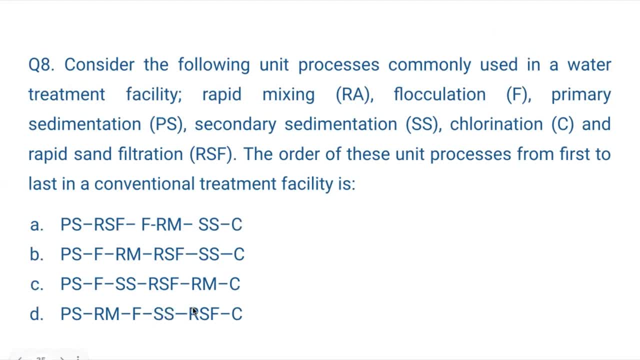 sanitation, then comes secondary sedimentation, and then comes rapid sand filtration and then comes inflammation. primary, primary sedimentation. first there will be primary sedimentation, then we will coagulate the rapid mixing of them- sorry, i still being recovered- completely by covering covid. then we will Favorby in tank that flo g früh. 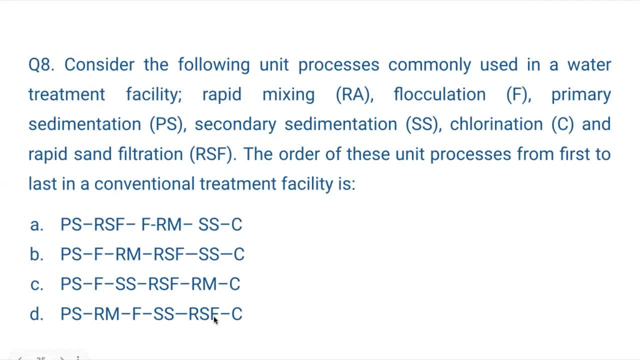 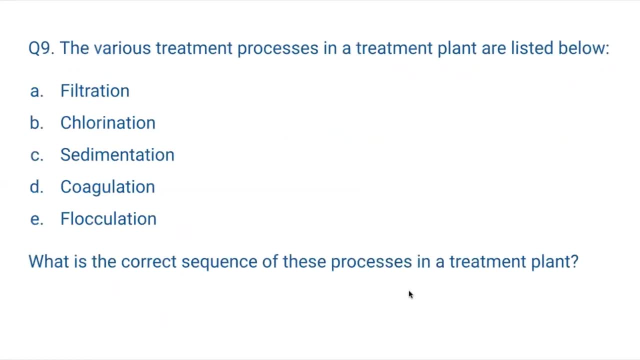 setter again, then there will be vlog then appear: walk nailed greater né rapids and filters it, filter, carrying on. finally, chlorination: connect with homes. go supply current would be. is the correct answer? question 9: the various treatment processes in a treatment plant are listed below: filtration, chlorination. 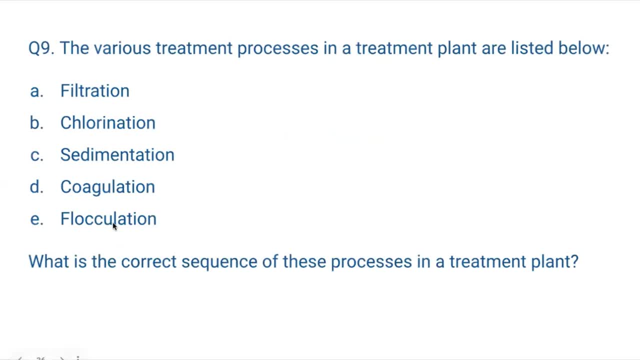 sedimentation, coagulation and flocculation. the same question, it hasn't just been flipped. what is the correct sequence, sequence of these processes in a treatment plant? but you shouldn't plant my in processes but cast his sequence hotel it both. the question number 8 and 9 is at the same but there. 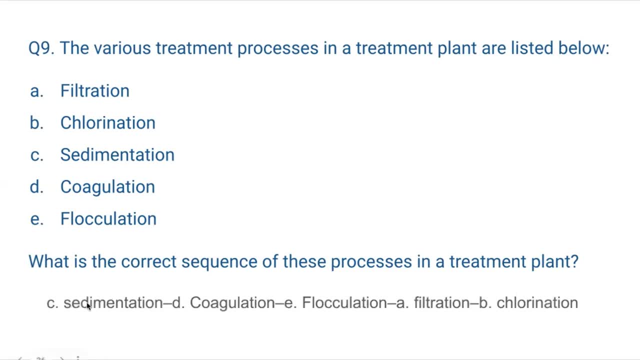 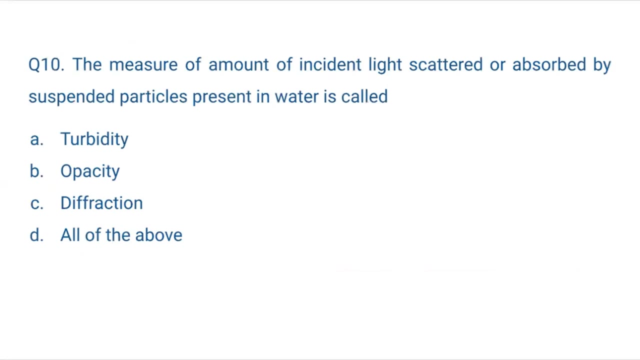 is a different way of asking these questions. we all know: first step, sedimentation, then coagulation, then flocculation, then filtration and finally coordination ticket. final question: the measure of amount of incident light scattered or absorbed by suspended particles present in water is called so, Joe, incident line. funny the part I was supposed to cut, scatter Hoga, which.